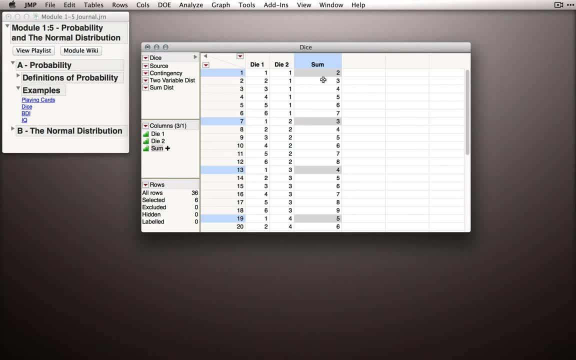 Now we're going to spend a lot of time talking about the probabilities of taking the sums of independent events. And remember, die 1 and die 2 are totally independent. So what we have here is a column that represents the sum of two independent events. Let's look at that distribution. I'll go. 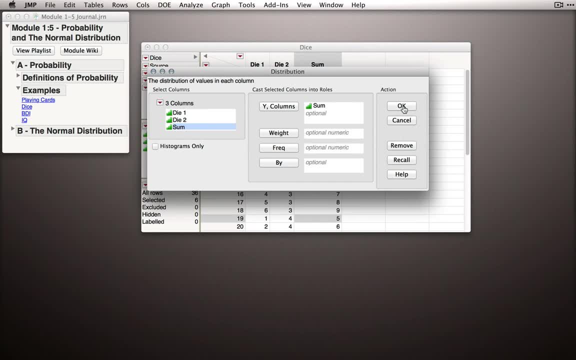 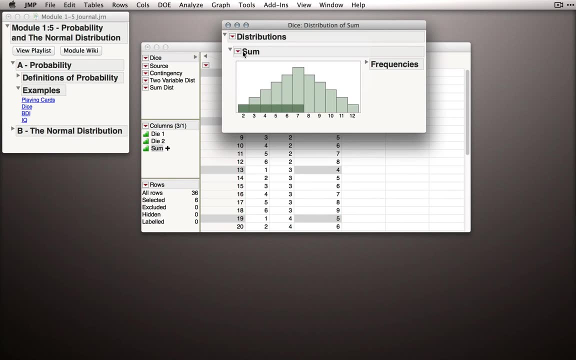 to Analyze, select Distribution and this time take the sum. I'll hide the statistical output and just to make things a little more clear, for this example, I'll go to the red triangle and stack. Remember, if you ever want your histograms. 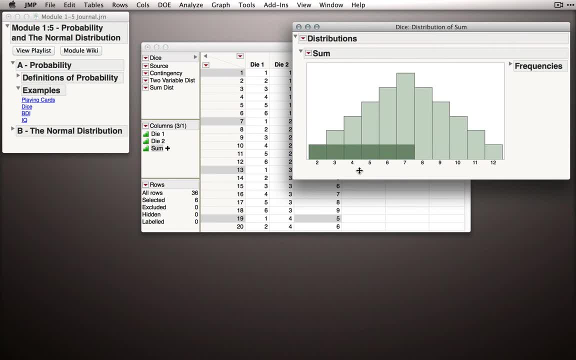 on the side. simply go to that topmost red triangle and stack the output. Let me clear my selection and let's just look at the distribution of sum. Now you might notice something here: Our original distributions, that is, the distributions of die 1 and die 2,. 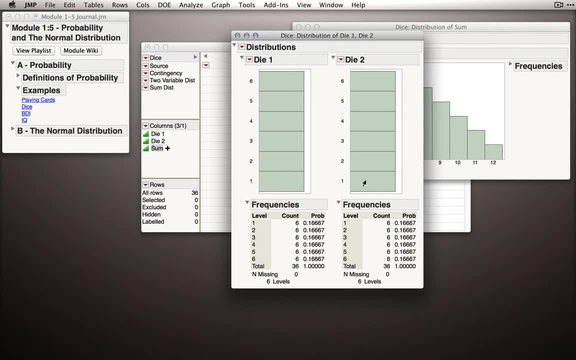 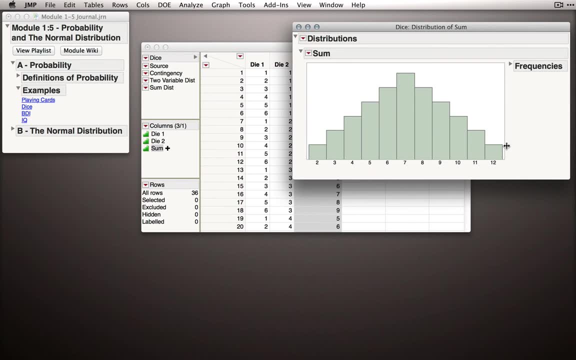 our individual rolls, for the first two die. those were completely flat, But as soon as we took a sum of the events, something happened here. Well, we can certainly see that the distribution is symmetric right. Our original distributions were 2, but we've actually ended up with a. 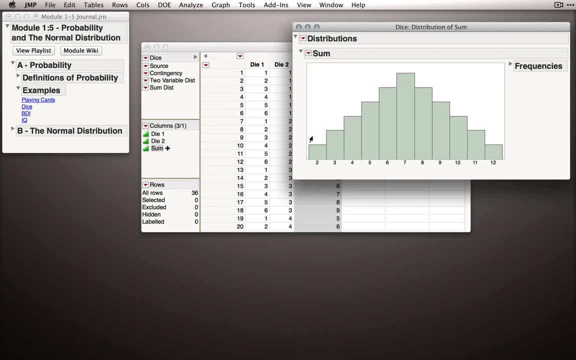 triangular shape for this distribution of the sum. Now that's interesting. Let's consider why we would get this shape. We can see from this distribution, like we can from any distribution that shows the probabilities of different outcomes, that the likelihood or the probability. 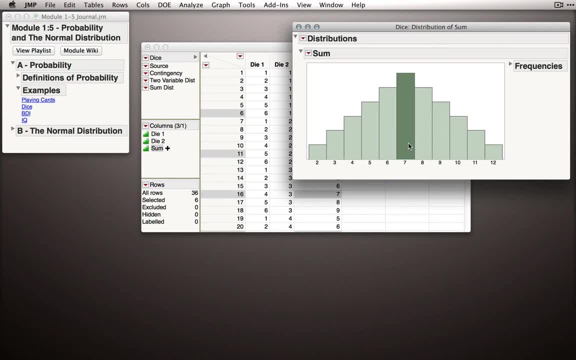 of getting a 2 or a 12 is much less than the probability of getting a 2.. And let's not forget what 7 here is representing. 7 here is the sum of the independent outcomes of die 1 and die 2.. That is, it is the sum of the number of pips showing up on each die. 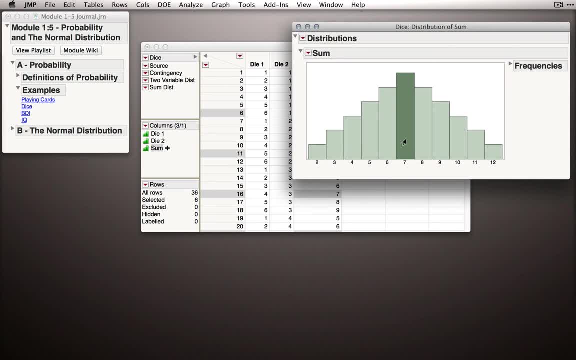 Now, how is it that we can get a sum of 7?? If you look in the dataset, you can see that we were able to get it six different ways. But let's actually look at those outcomes. I'm going to go to 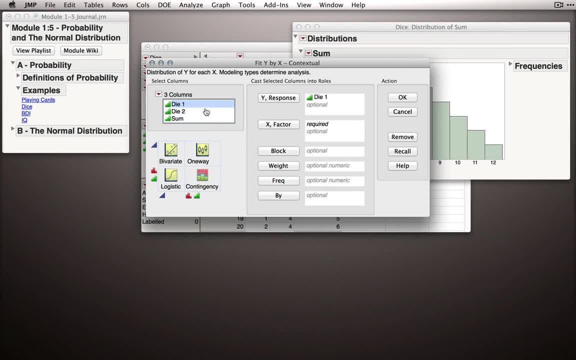 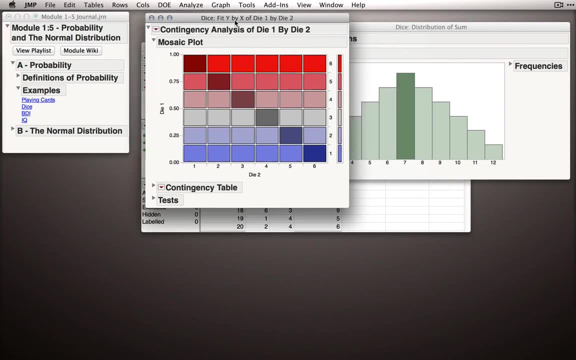 analyze, fit y by x again and put die 1 as my y response and die 2 as my y response Again. let's hide the statistical output and let's just look at what is shaded whenever we select these different outcomes. When I select 7, you can see this is the main diagonal of this.